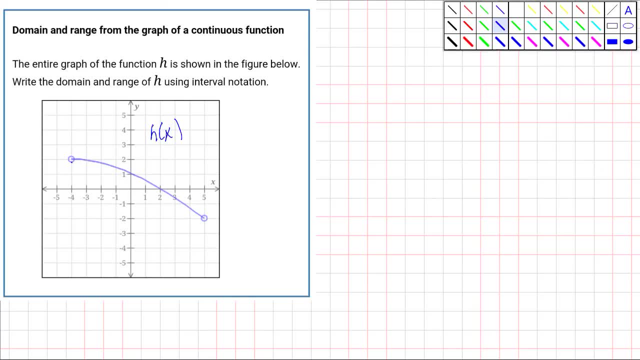 all the possible x values where the function exists. So when we look at the domain, we have to see that all the x values go from negative 4 to 5.. So the domain we have from 4 to 5, but then we have to look at 4.. At 4, do we have an open circle or do we have a closed circle? If we have, 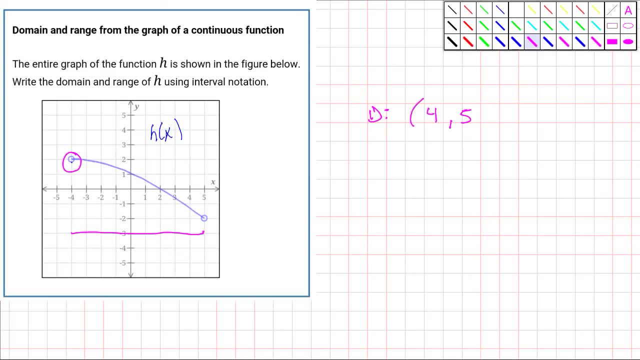 an open circle, then we have a parentheses. If we have a closed circle, then we would have a bracket. We look at 5, and 5 also goes from. it also has an open circle, so it also has a parentheses. Then I look at the range. 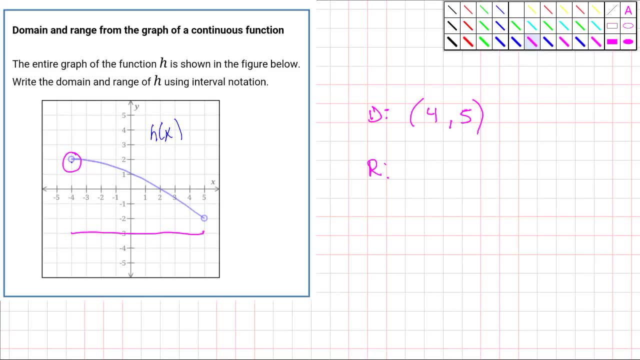 If I look at the range, I have to look at the y values. So to look at the y values I have to. so the function basically starts here and it goes all the way up to here. So that value is negative 2, right, That's the corresponding y value. So negative 2 and the corresponding y value. 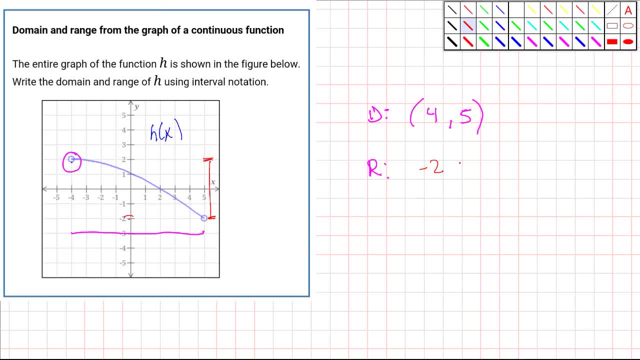 is. it goes all the way up to 2.. Now we'll look at negative 2.. Negative 2 is an open circle, so we have a parentheses. 2 also corresponds to an open circle, so we put a parentheses. So when we look at here, right, we have negative 4,. 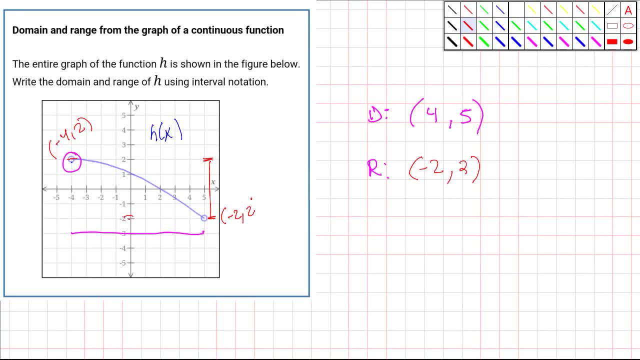 we have a point over here. we have negative 2, comma. I'm sorry we have. we have 5, comma, negative 2.. So we have 4, 2, and yeah, that's right. So when we look at this, 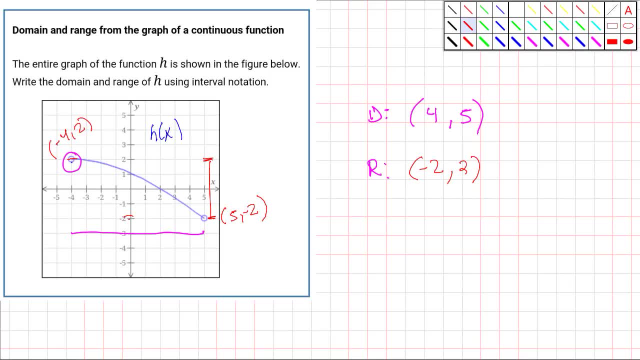 that's, that will be the domain and the range of the function. Now, how would this change if, let's say, you have a problem and you have a problem, and you have a problem and you have a? let me just do so. I'm going to do it on the same graph. 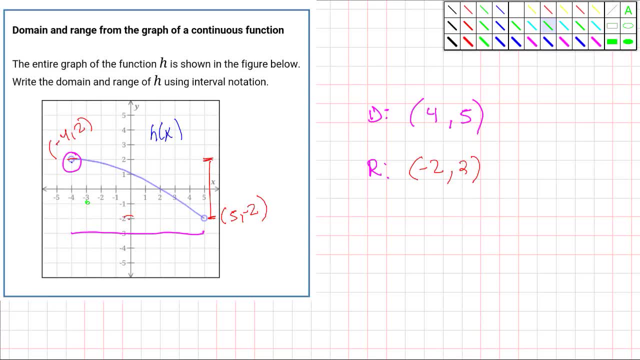 so I don't have to. So let's see if I have something like this right. and it came down like this. So to look at the domain, how the domain, I say: okay, the function on the x-axis spans right from negative 3 to 5.. So the domain, I say, goes from negative.